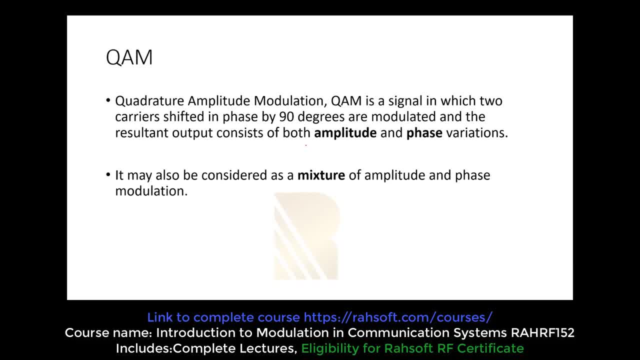 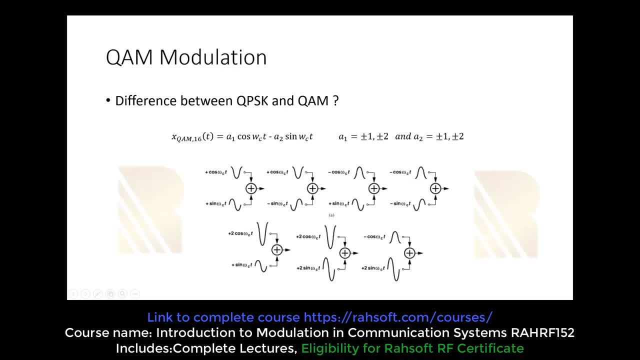 considered as a mixture of amplitude and phase modulation. It means that this time we are not only changing the phase, but we are also changing the amplitude. So, in order to understand the QAM, we are going to have an easy comparison. So we are comparing QPSK and QAM this time, So this is an easy level. 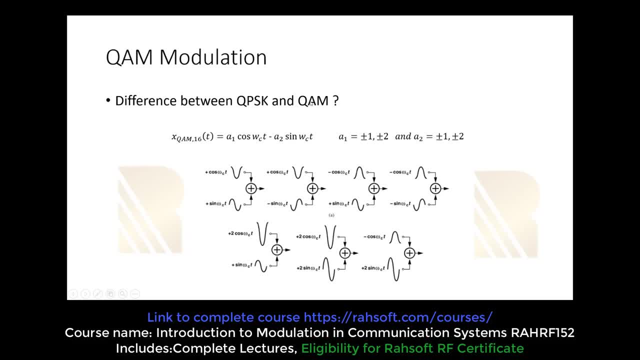 of QAM. It's not the only level. We are going to have 8 QAM, 16 QAM, like other ones, but this is the basic levels. So let's see what is happening. For QPSK, we said that the output is A cosine omega Ct minus A2 sine omega Ct, So let's review. 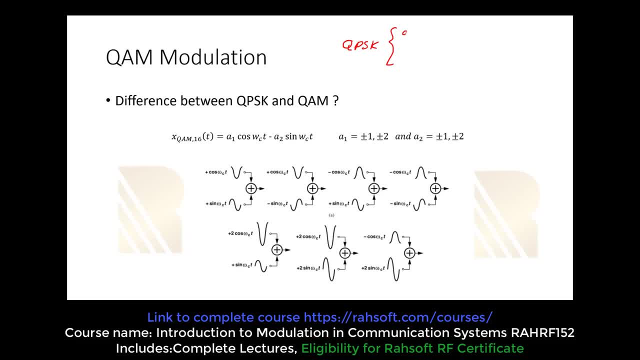 this For QPSK. we said that the A1 and A2 we have, or A, B, and there are different definitions. It doesn't matter. I'm going to show with A1 and A2.. Or you can also call it I and Q. So A1 was plus and minus 1, and A2 was plus minus 1.. So 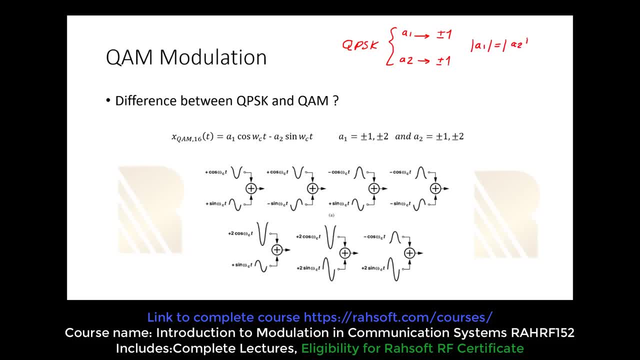 the absolute value for A1 was equal to A2, and that's why we said: the amplitude is not changing in QPSK, So we are only changing the phase. But the new thing includes the amplitude. So the amplitude is not changing in QPSK, So we are. 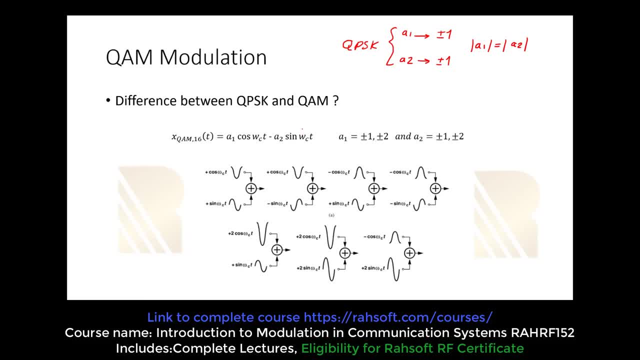 changing the amplitude. So QAM is this time we are also changing the amplitude. As you see, in the new system in QAM or QAM, the A1 is going to have two values: plus and minus 1 and plus and minus 2, and for A2 as well. So we are going to 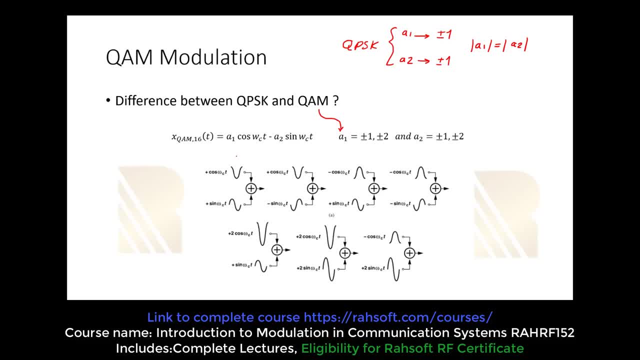 have this kind of things at the output. So, if you remember, this was our I part and this was our Q part, and then they're the same for other pictures too here. So here let's say we have 1, 1, cosine sine, cosine minus sine. So up to here. 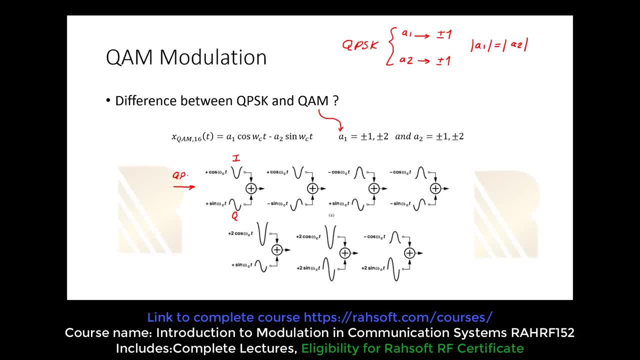 the top one here is actually QPSK. yeah, because we have the same amplitude level, But these in the bottom they're showing the new waves for QAM, And this time we are going to have 2, 1, 2, 2, minus 1, 2, and there are more even because we can have different things. 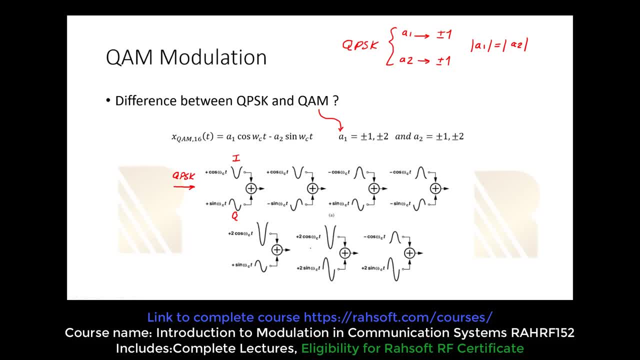 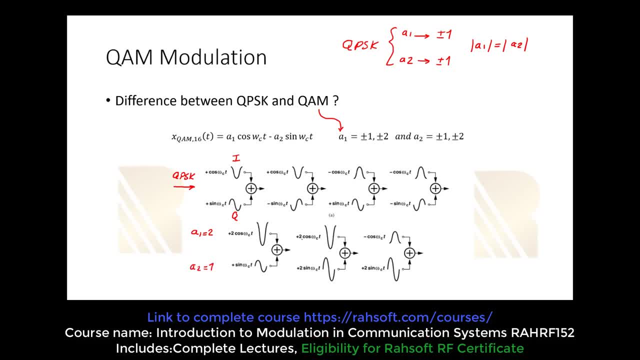